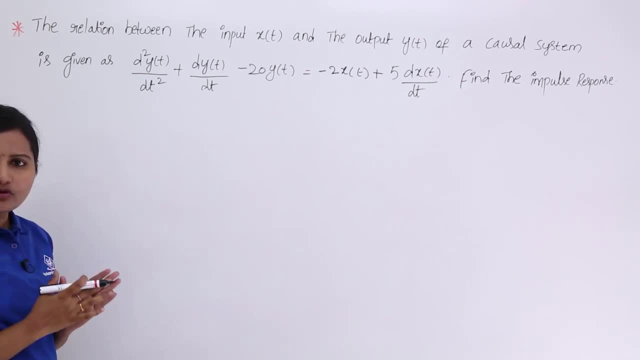 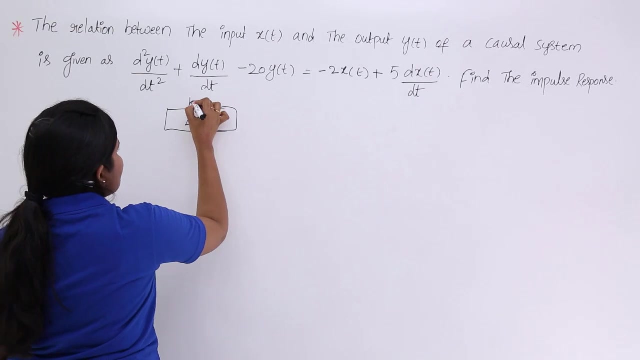 out the impulse response. Whenever you are hearing about input, output and impulse response, you need to think about LTI system. So we know about LTI system. for example, if you are having any LTI system with impulse response h of t, this system is excited with a. 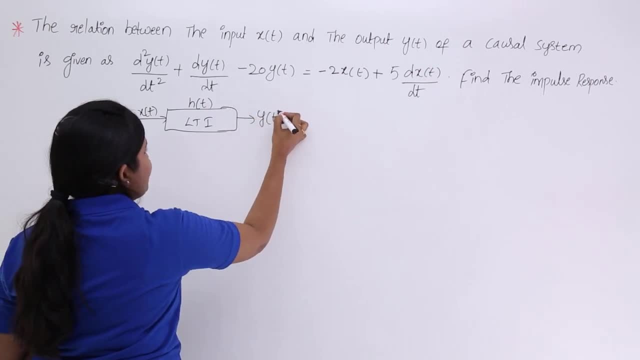 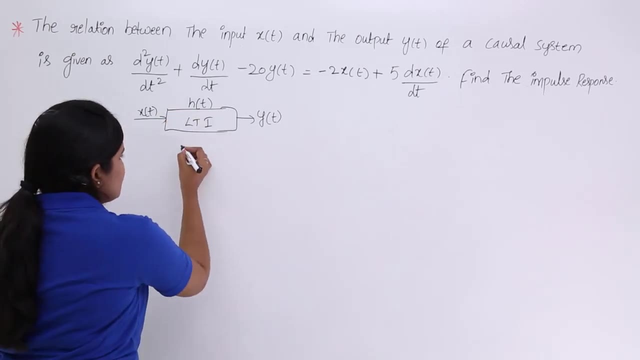 signal x of t and this system is producing response y of t. the relation between output, input and impulse response will be like this: The output of LTI is equivalent to input and impulse response. So you need to think about LTI system. So we know about LTI. 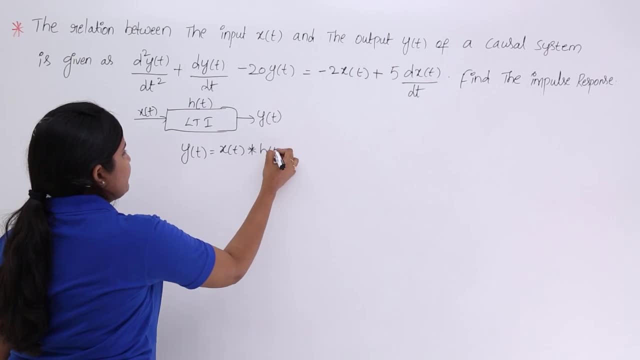 and output, input convolution with impulse response. Now same equation we can write in frequency domain, as y of s is equal, into x of s, multiplication with h of s, where h of s is the transfer function of the system And that means convolution. 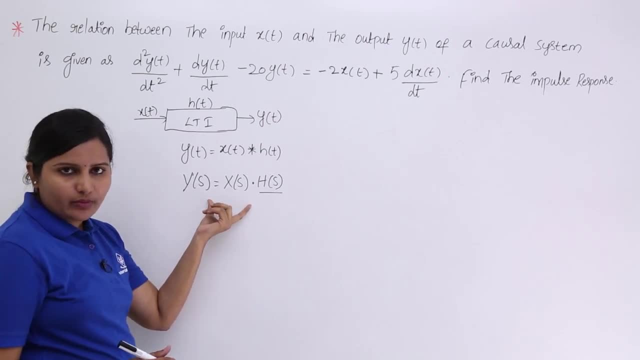 in time domain leads to multiplication in frequency domain. So here they. given the relation between us, this system urban gone. So you look at another example where you havelied an escaping of time flight n, And then here you have 12 t times n, 1 x probation. 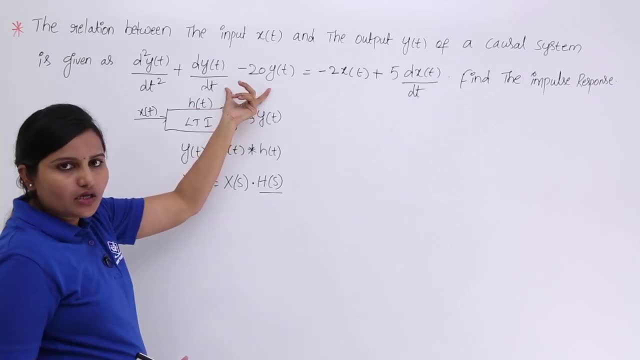 of y of t and x of t by using this differential equation. So by using that you need to find out x of h of t. but if you are using this equation that is typical to find out h of t, why? because it is typical to separate convolution to get h of t. 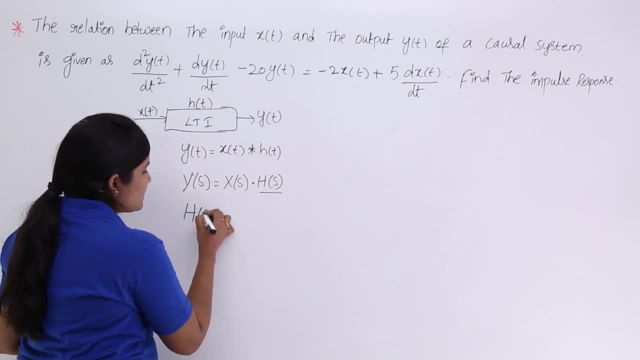 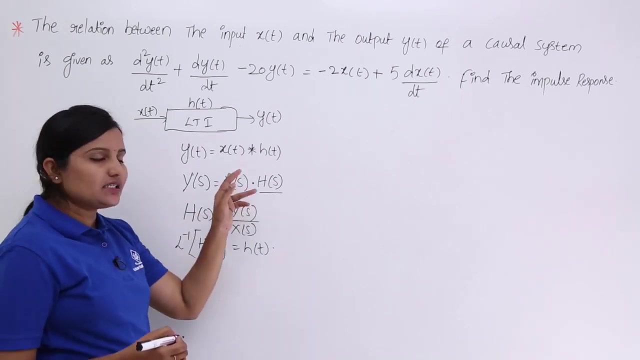 But here, if you are doing like this, h of s is equal into y of s by x of s. that means, if you sent x of s this side and if you consider inverse Laplace transform of h of s, simply you are going to get h of t. So here, as this transforms in multiplication, then it is easy. 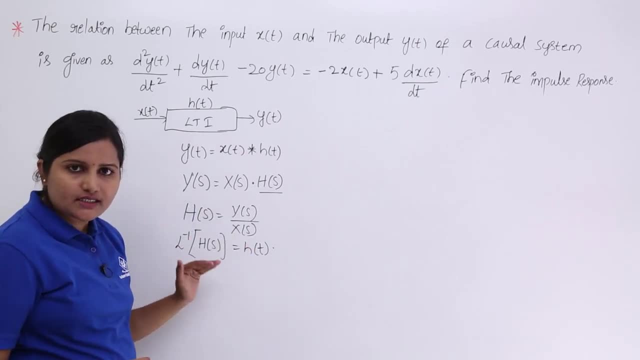 to find out the transfer function. by the transfer function it is very easy to find out the impulse response of the system. So this process I want to execute now. that means I want to follow my process in frequency domain, not in time domain. So here I am going to do the same thing here. So here I am going to do the same thing here. 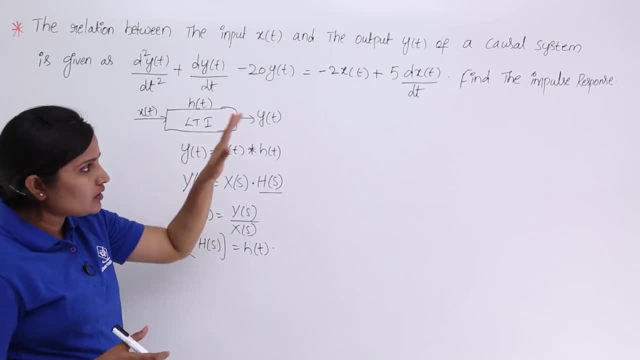 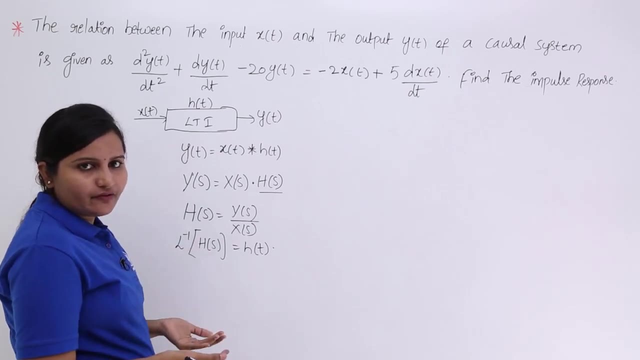 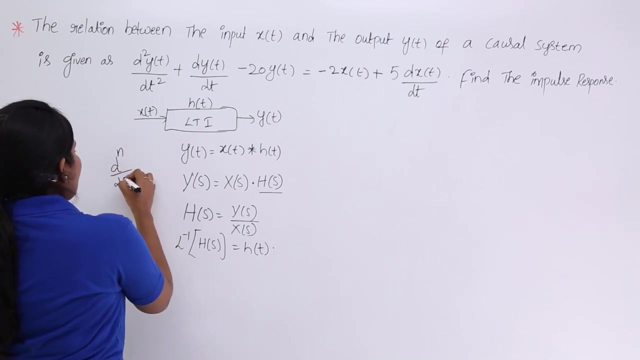 So here I am having this differential equation. before going into the procedure, I want to discuss with you one thing about differentiation property. We already discussed differentiation property in Laplace transform, that Laplace transform of d power n by dt power n into x of t is having Laplace transform s power n into x of s. So that means, if you are, 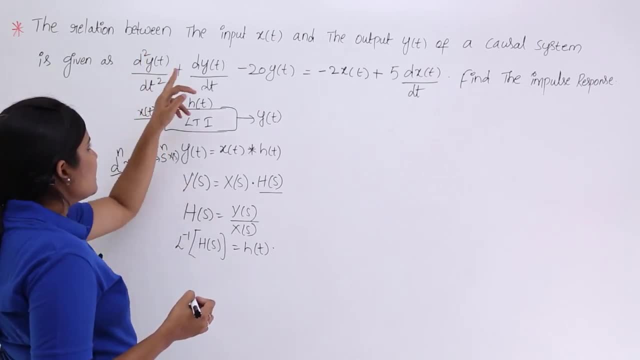 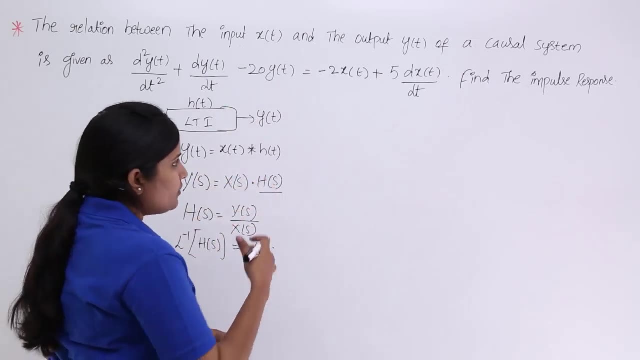 having d square, then you will get s square into x of s. If you are having d, then s into x of s. For example, if you are having y of t means you will get y of s. Now, by writing, you can understand. I am going to consider this differentiation. 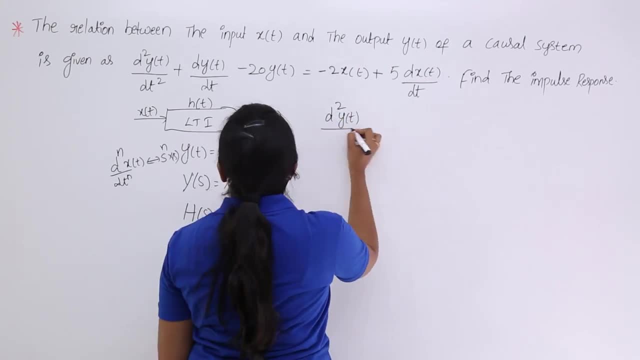 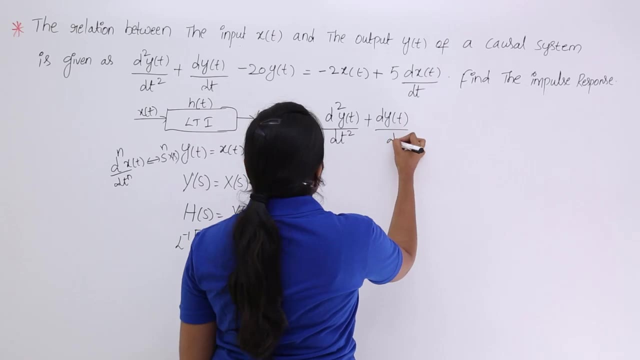 equation as it is, this differential equation as it is: d square y of t by dt square, plus dy of t by dt, minus 20 y of t is equivalent to minus 2 x of t plus 5 dt square, and I am going to write that just to Sy, okay, So here we are, generating Y of t, of y is equal to: minus y. the first thing that I want to do here I am taking X of t from X square called minus T. y of t is equal to minus 1Y of t. plus Y of t is equal 2 X of t. this way, all letters. 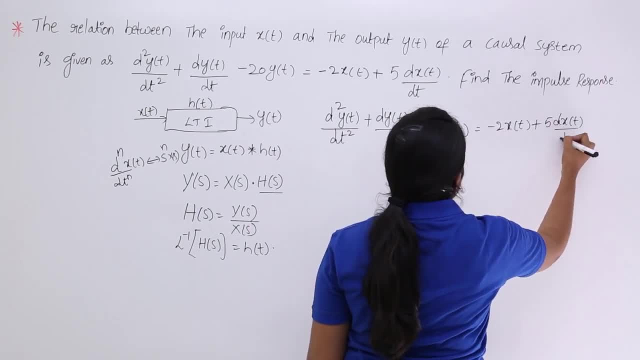 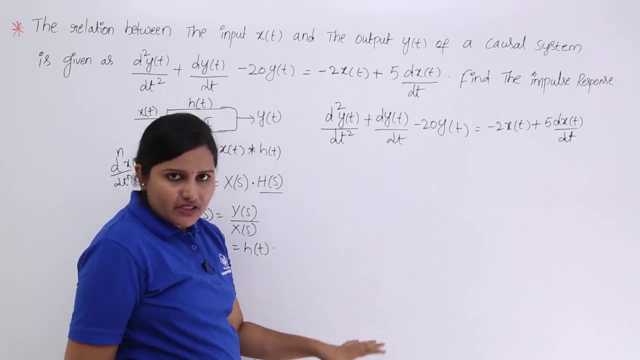 will be written Y of t minus T, y of t. the first letter is Y of t, that is the fruit of Laplace. transform dx of t by dt. Now you can see, I want to propagate my problem in frequency domain, not in time domain. I want to solve my problem in frequency domain. So here the problem given. 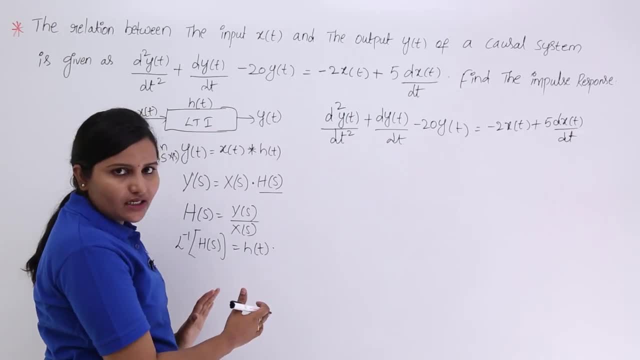 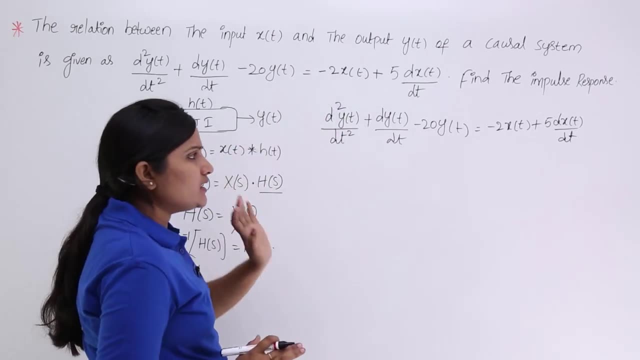 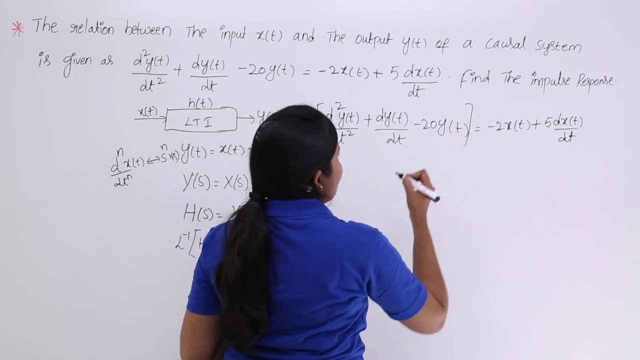 is in time domain. by this knowledge, I understood that it is very easy to solve this same problem in frequency domain. So now this is in time domain. means how we can convert time domain into frequency domain. means by taking Laplace or Fourier transform. now we are taking Laplace. 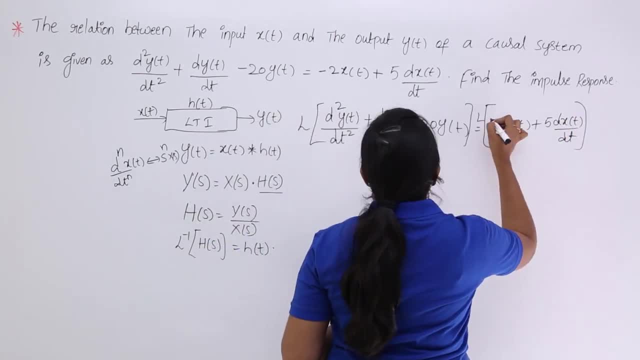 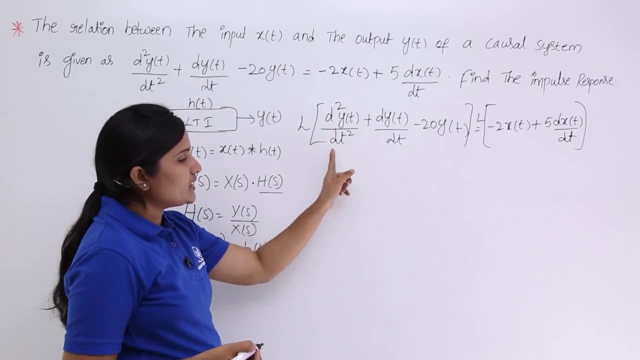 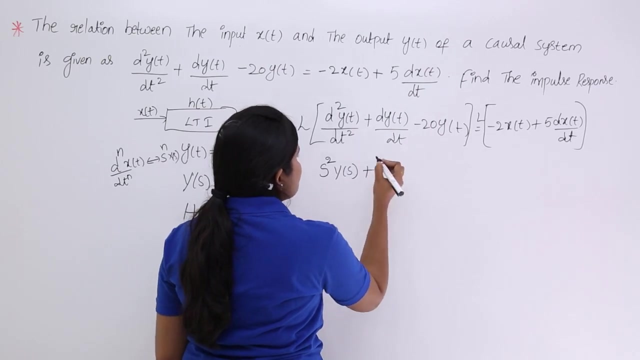 transform. So here I am taking Laplace transform on both sides. If you are taking Laplace transform on both sides. Laplace transform of d square, y of t. by dt square according to differentiation property, you can write s square into y of s plus. here. Laplace transform of d, y of t. 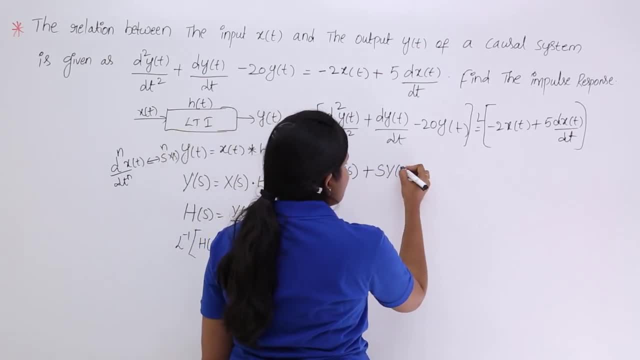 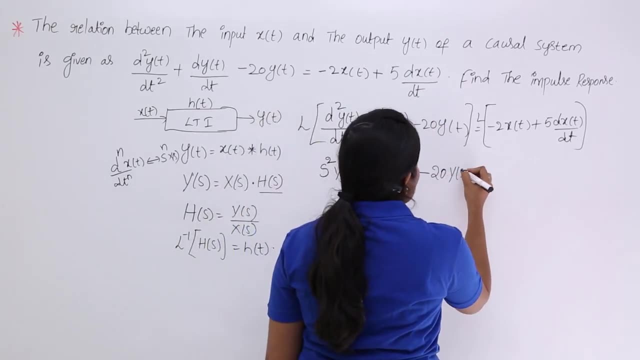 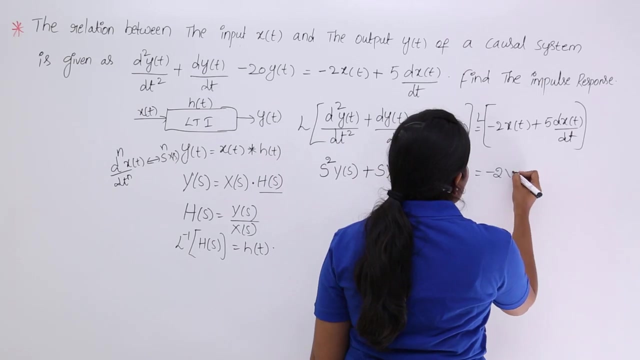 by dt. you can write like: s into y of s. Minus Laplace transform of 20 into y of t. you can write like: 20 into y of s. this is equal into Laplace transform of minus 2 into x of t. this can be written as 2 into x of. 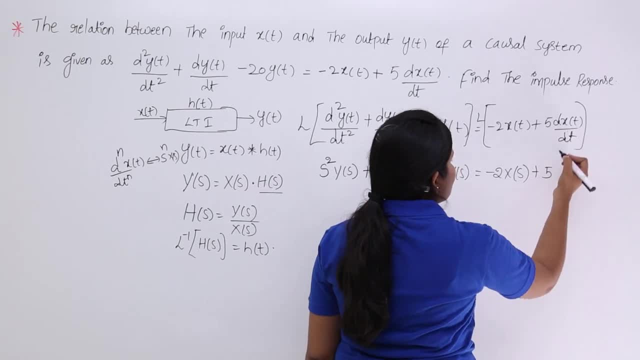 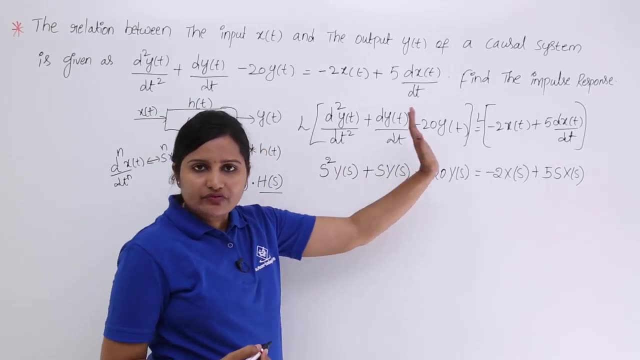 s and plus. here we are having another differentiation: So s into x of s. So like this we need to write the Laplace transform of this differential equation: hand side: we are having common of y of s. I am going to take the common of y of s here. 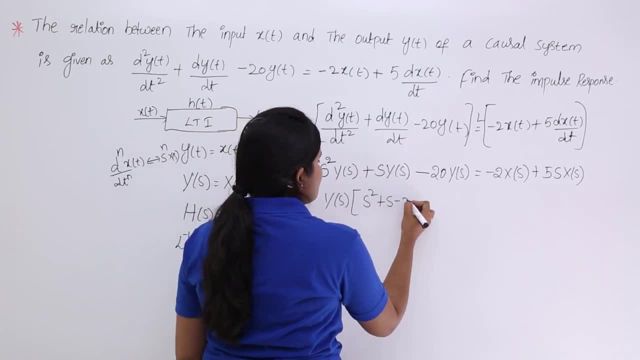 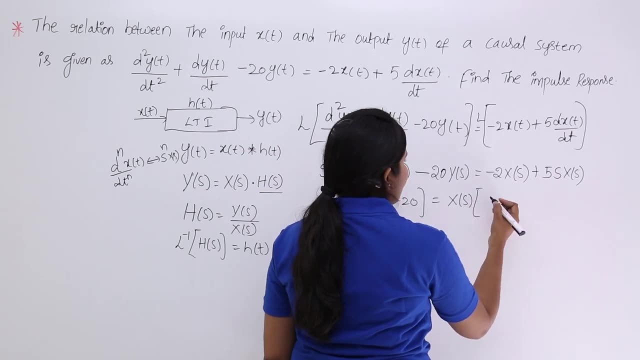 y of s into s square plus s minus 20 is equivalent to this side, I am having common of x of s. If I take in common of x of s, I am going to get 5s minus 2.. So see, here we are very near. 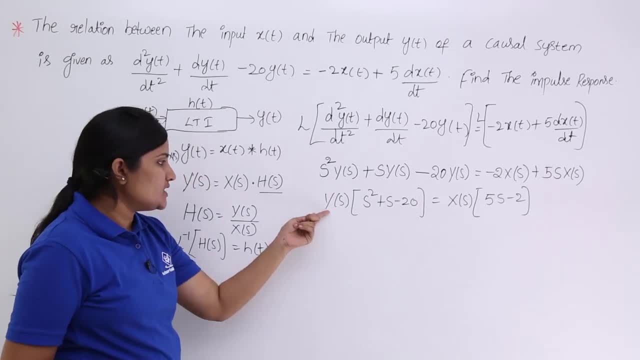 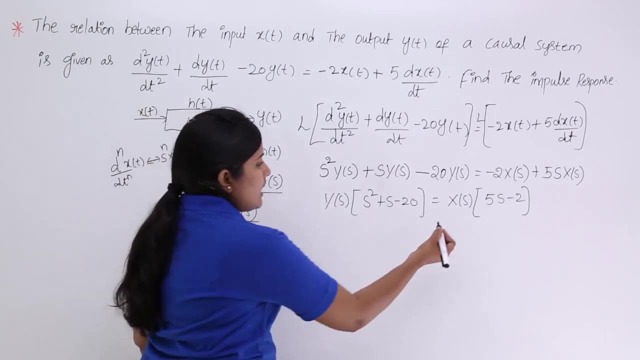 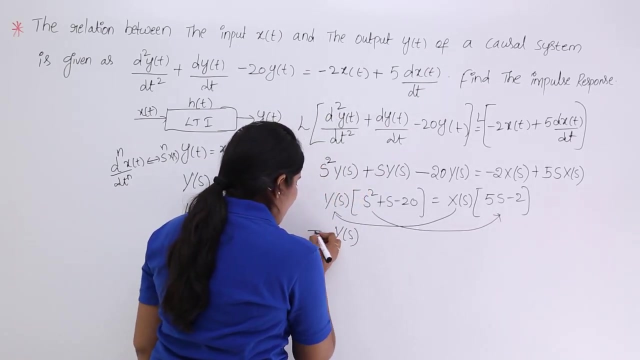 to h of s. if you send this x of s to this side, So that will become y of s by x of s, then we can say that is equivalent to h of s. I am just sending this to this side, and I am sending this to this side, So y of s, that implies y of s by x of s, is equivalent. 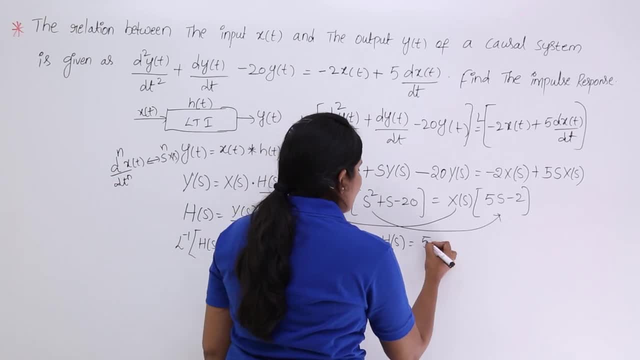 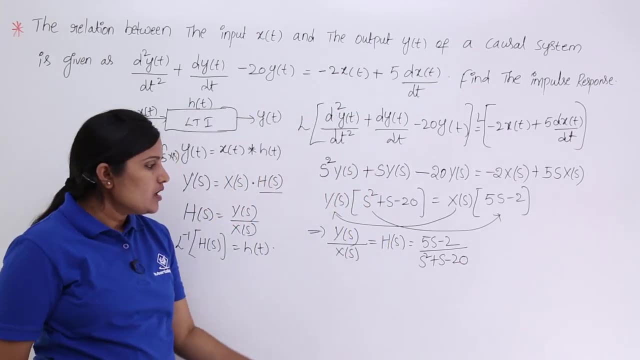 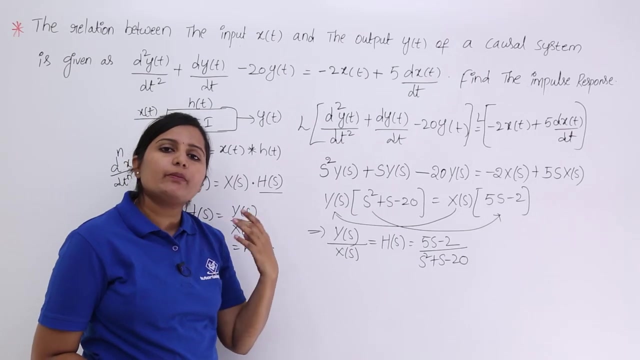 to nothing. but h of s is equivalent to 5s minus 2 divided by s square plus s minus 20.. Ok, Now our h of s is ready. but how we can consider inverse Laplace transform? So definitely, we can take this directly in inverse Laplace transform equation. but if you want to apply, 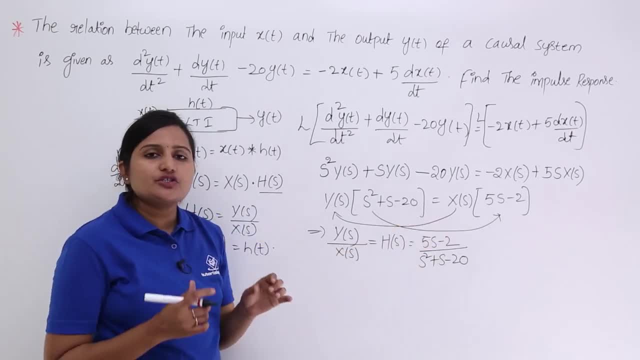 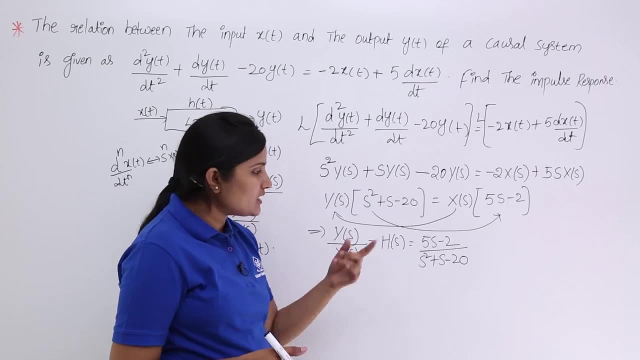 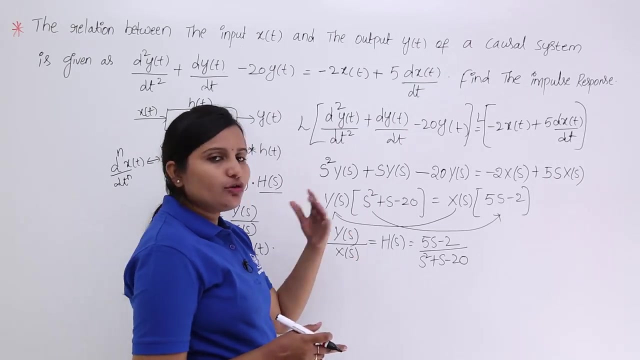 shortcut: Laplace transform pairs. your equation should be in the form of standard pairs. So here, by observing this equation itself, we cannot say that is in some Laplace transform pair form, So this is not in any transform pair form. So we need to make that in any one of the 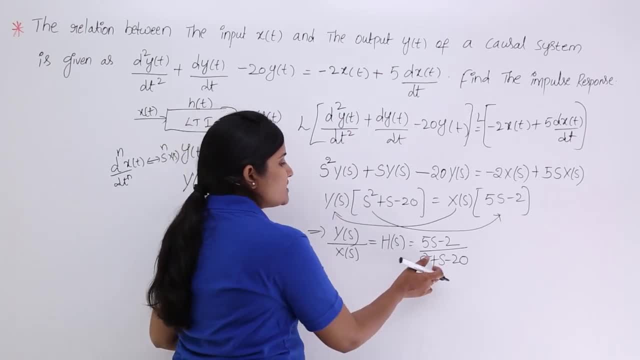 standard transform pairs form. So further I want to consider the factors for the denominator. like 5s minus 2 divided by So this one, how we can write, means 4, 5s 20.. So 4, 5 minus. 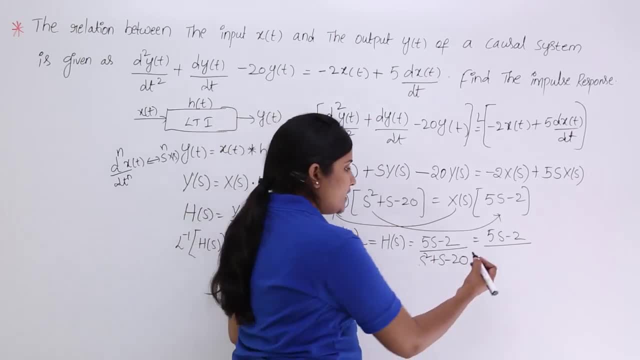 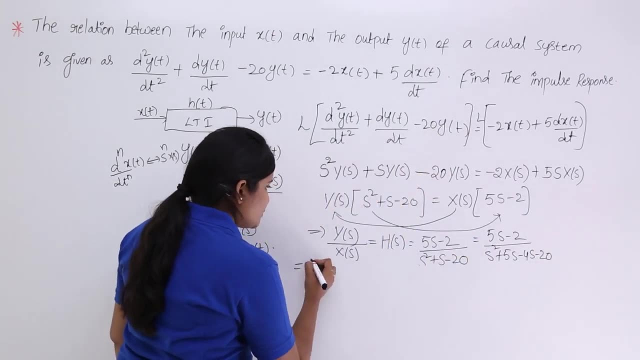 4 1, we will get 1.. So I am writing like this: s square plus 5s minus 4s minus 20.. So this is equivalent to 5s minus 2 divided by s square, or s you can take common s into s, plus 5 minus. 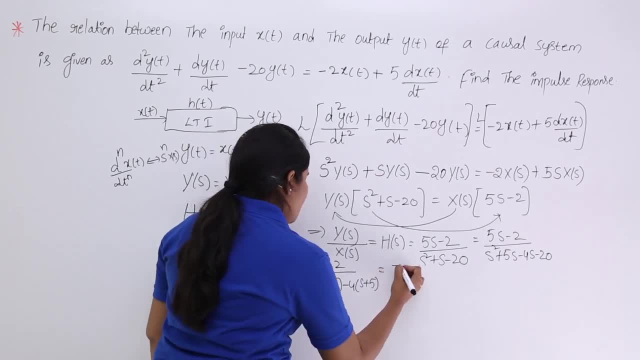 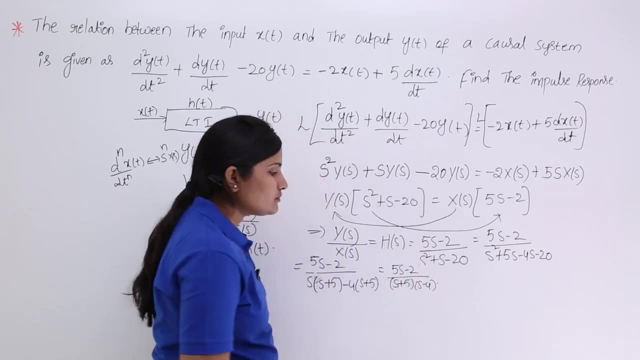 4 into s plus 5.. So you can say 5s minus 2 by s plus 5, and s minus 4 are the factors. Now, if you consider partial fractions, then that will be the fact. Summa cum, SAY i: 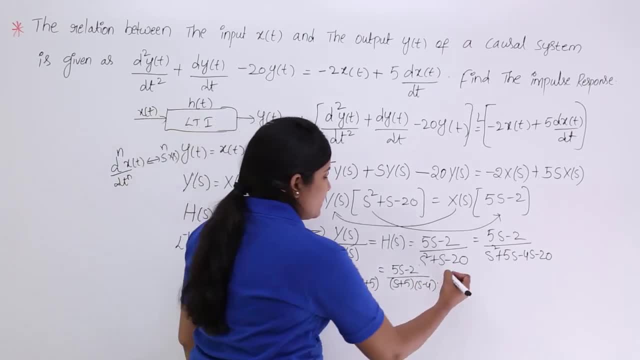 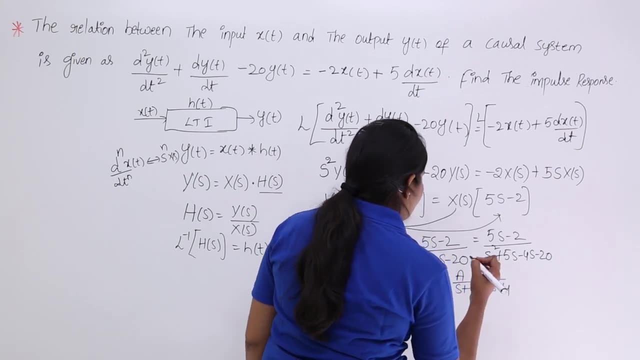 C: 1, 7, 8, 1, 1, 3, 12, 16, 20, 15, 75, 27, 51, 60, 70. that is equivalent to a by s plus 5 plus b by s minus 4.. Then what will happens So? 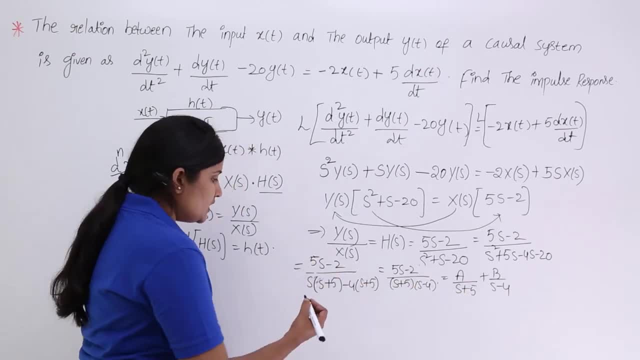 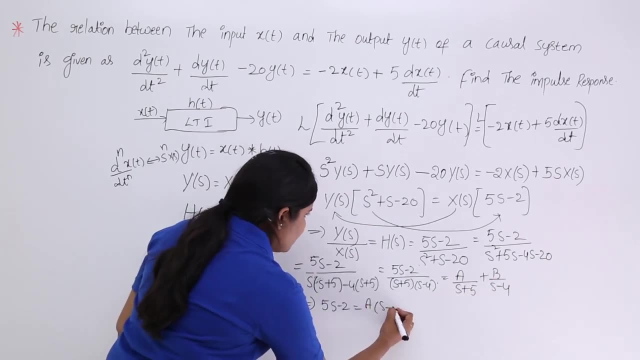 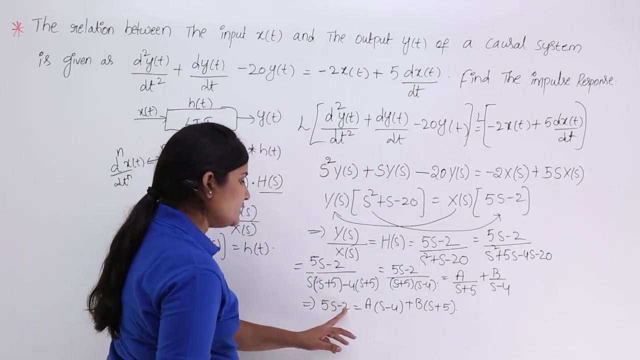 if you, if you consider partial fractions, then you can write like this: 5s minus 2 is equivalent to a into s minus 4 plus b into s minus s plus 5.. I am just comparing the constant terms. If I compare the constant terms, minus 2 is equivalent to minus 4 a plus. 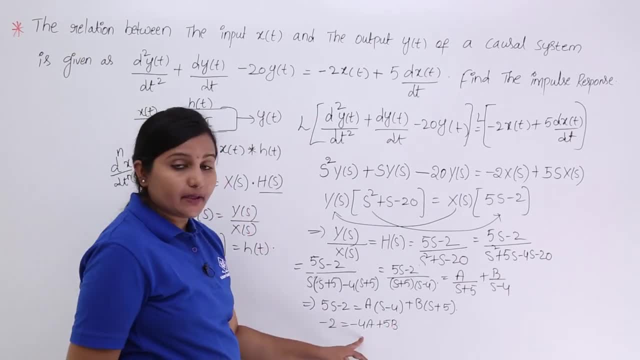 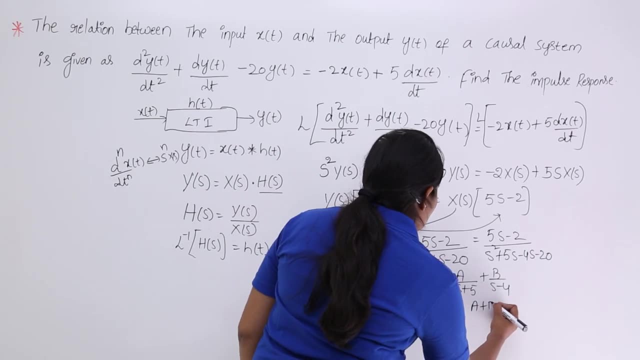 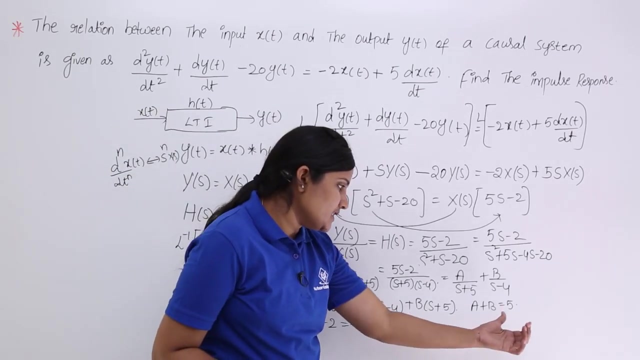 5 b minus 4, a plus 5 b. If I compare the s terms, a plus b is equivalent to 5, a plus b is equivalent to 5.. So if I substituted a is equivalent to 5 minus b. if you calculated. 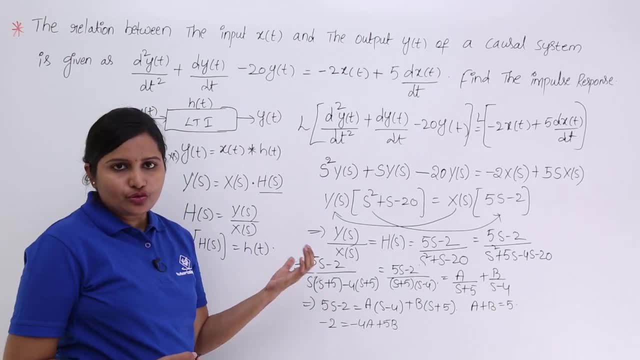 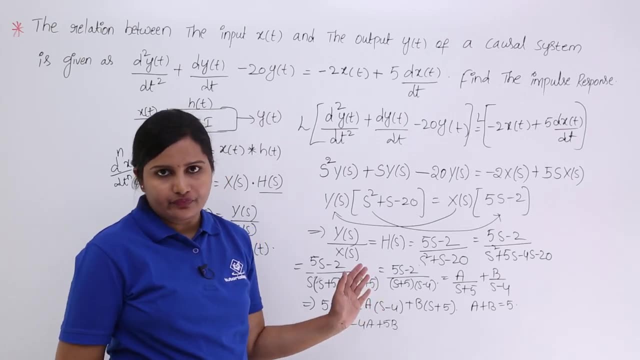 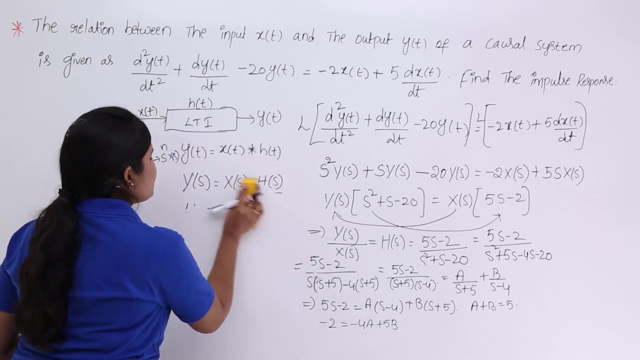 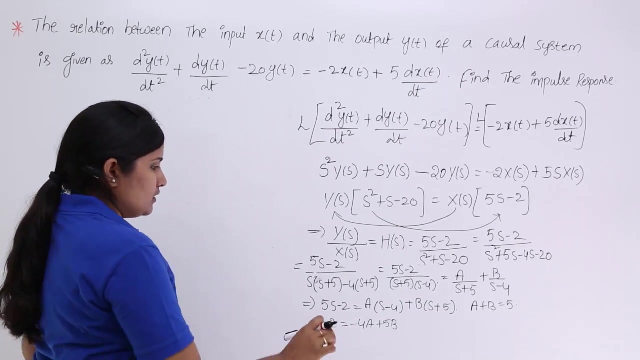 this: You are going to see that you are going to get 2 as your b and 5 as your a. So here, in place of here, I want to calculate that, So I am going to rub this. If you want to calculate that, then see that we got two equations. 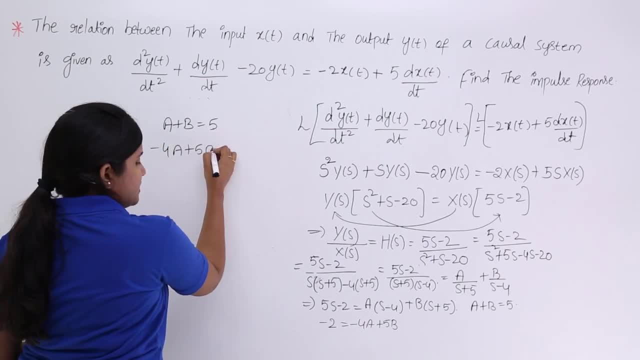 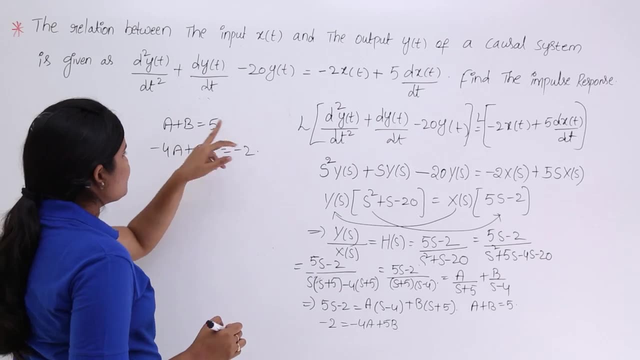 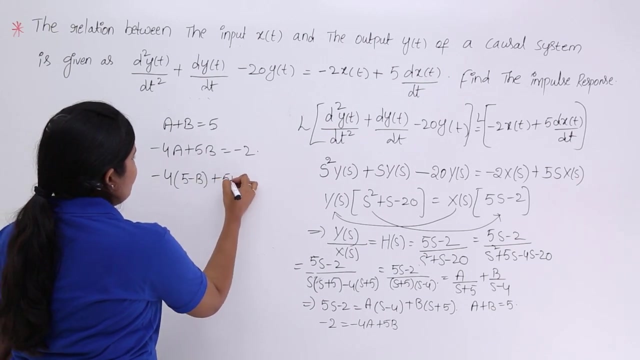 4 a minus 4 a plus 5 b is equivalent to minus 2.. Here in place of a I can substitute 5 minus b. So in place of a I can substitute 5 minus b. plus 5 b is equivalent to minus 2.. So here: 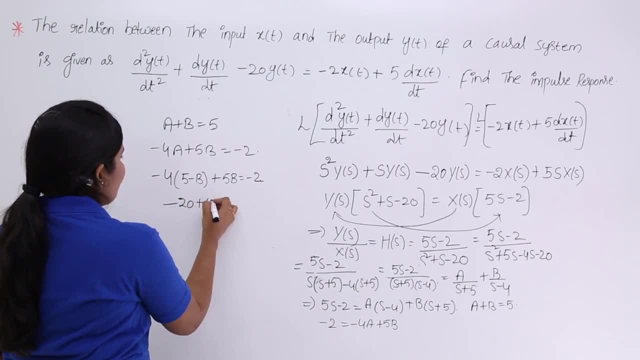 you can see: 4- 5 is 20 plus 4. b plus 5 b is equivalent to minus 2.. If I send this 20 to this side, you are getting 4 b plus 5. b means 9, b is equivalent to 18, 9- 2s, So b is equivalent. 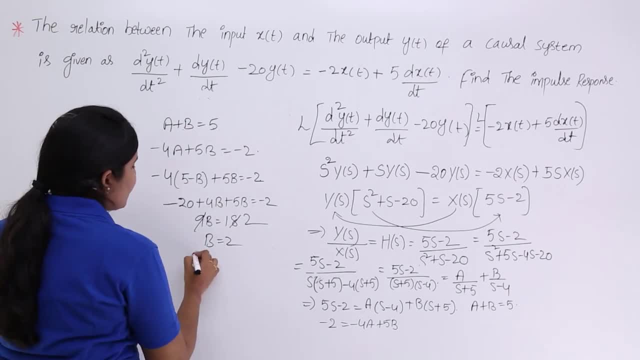 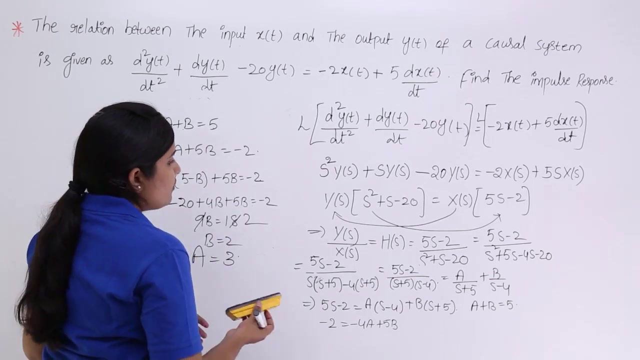 to 2.. And if you substitute this 2 here, you are getting a is equivalent to. if you substitute b is equivalent to 2 here, that 5 minus 2, you will get a is equivalent to 3.. So you can write from now onwards, you can write your h of s as h of s. this is your h of s. 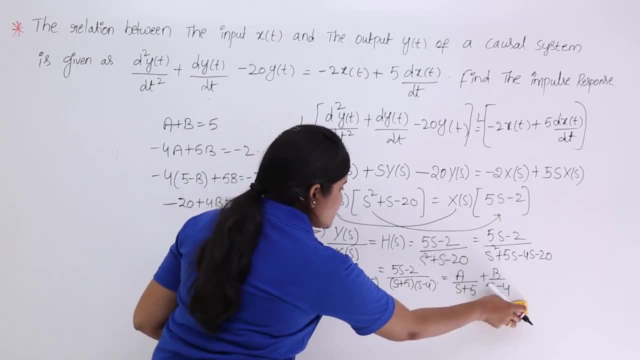 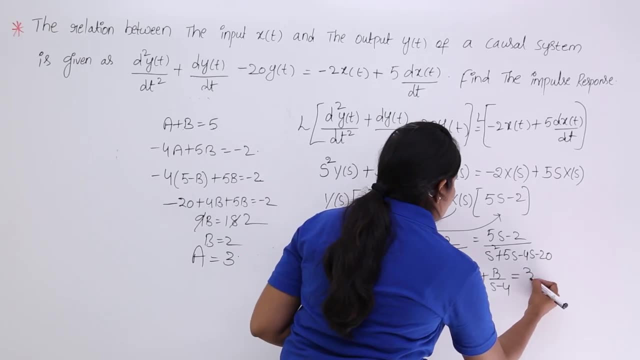 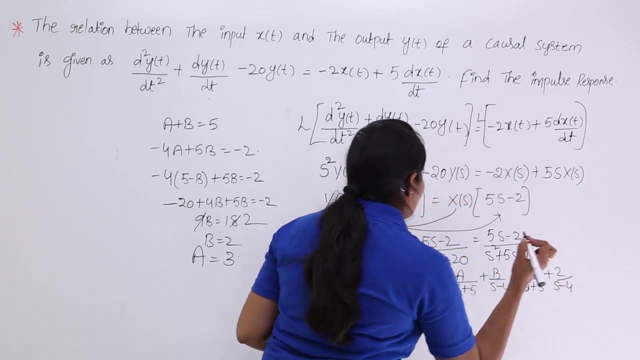 right. So up to here, this is your h of s. So now you can write your h of s as a value is equivalent to 3, 3 by 5 s plus 5 plus b. value is 2, 2 by s minus 4.. This is your a. 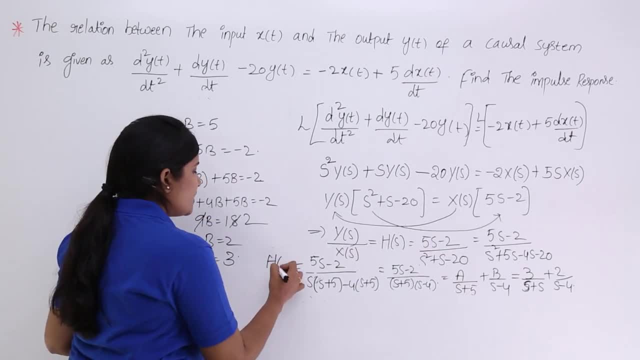 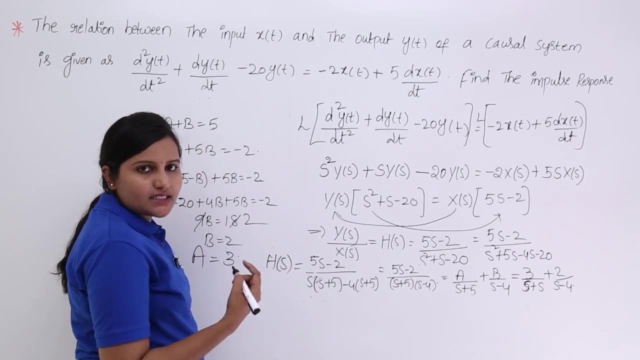 and b values, H of s. but we do not want H of s, we need H of t. So how we will get H of t from H of s: by just considering inverse Laplace transform. we are going to get H of t. That means by: 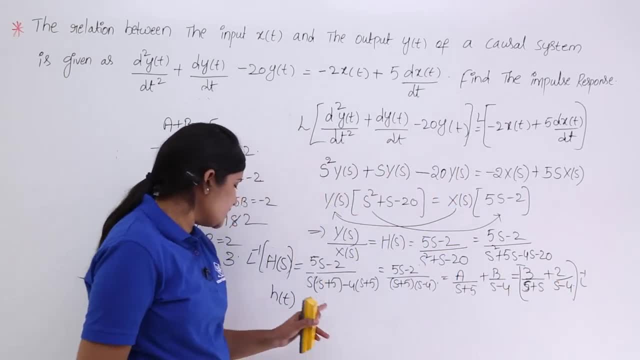 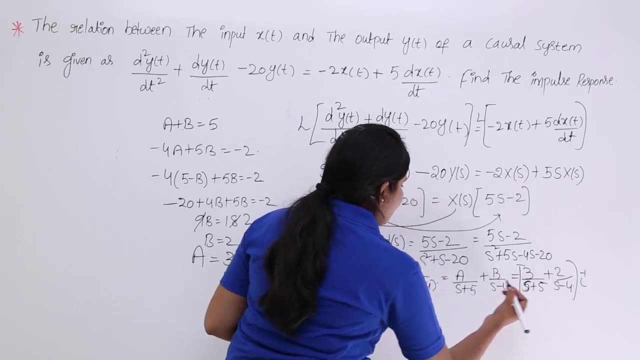 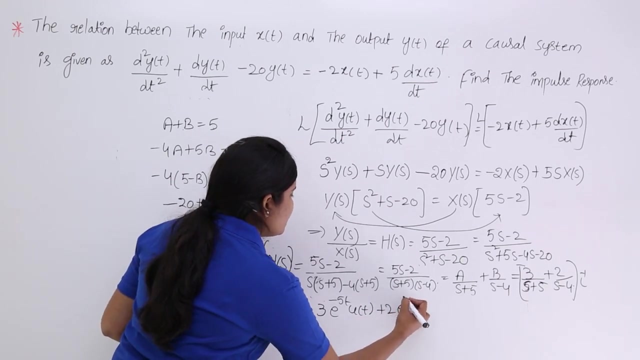 taking inverse Laplace transform, we are going to get H of t, So H of t is equivalent to 3, is constant, 1 by s plus phi, So 1 by s plus phi. you can write like e power minus phi t? u of t plus 2 into e power plus 4 t minus 4 t? u of t. So this one plus means 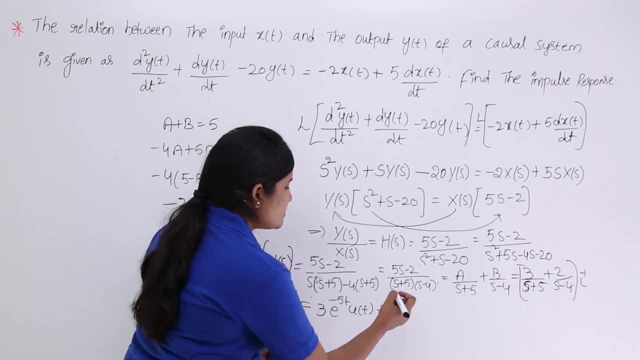 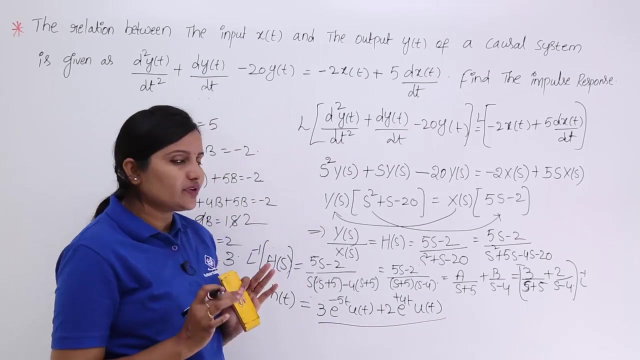 so e power minus phi t u of t. So here minus means plus 4 t u of t. When you are having minus here, you need to consider plus in the exponential. when you are having plus here, you need to consider minus in exponential. This is the impulse response of the system. 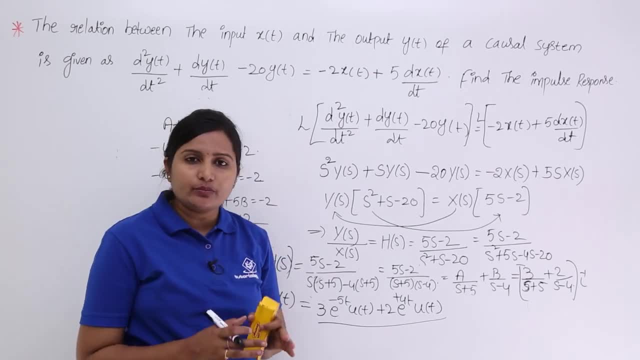 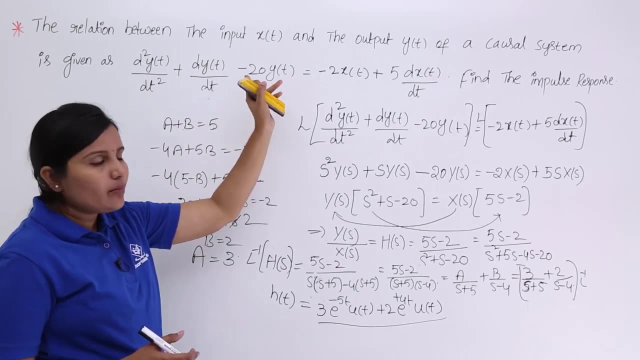 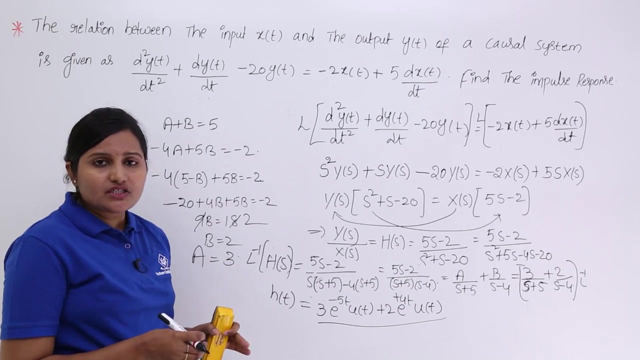 whenever you are having. So you are having the relation between the input and output as a differential equation stating: d square y of t by dt square plus dy of t by dt. minus 1 t y of t is equivalent to minus 2 x of t plus phi dx of t by dt. If this is the differential equation stating 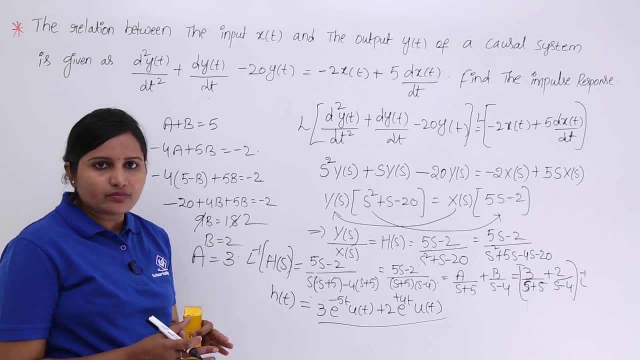 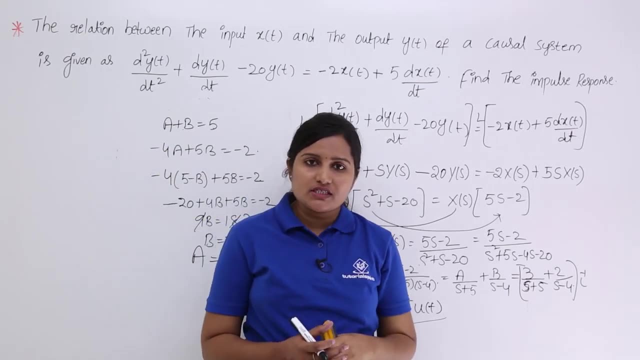 the relation between input and output response of a system. the impulse response related to the system will be like this: Like this way, we need to solve impulse response of the system by using differential equation: differential equation relating input output response.